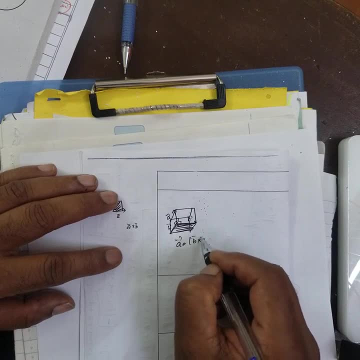 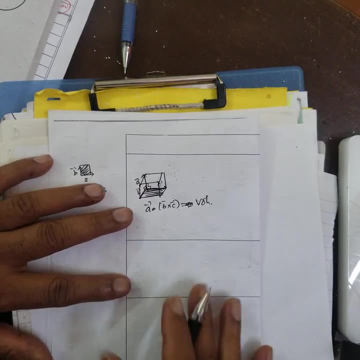 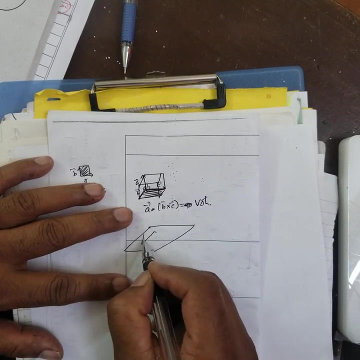 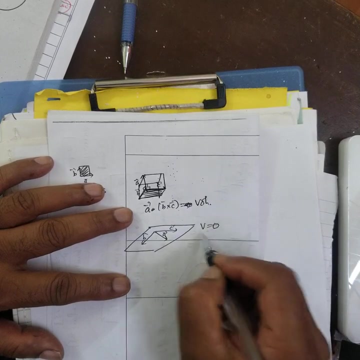 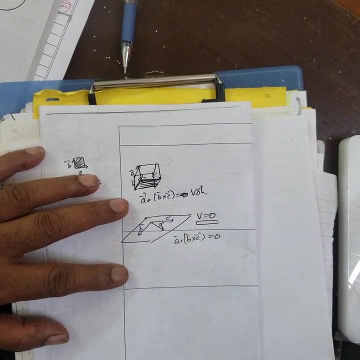 A, dot, B, cross, C, C equal to zero. Sorry, this is volume, Volume of the parallelepiped. Suppose: if there is a plane Here, B is here, C is here. If A falls on this, If A falls on this, volume becomes zero. What is volume becomes zero. That means A, dot, B, cross, C is equal to zero. That means scalar. 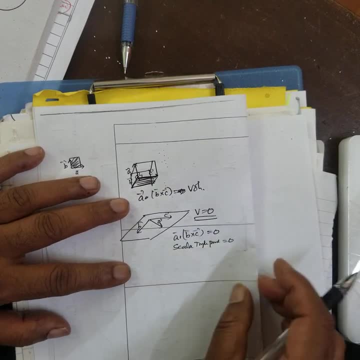 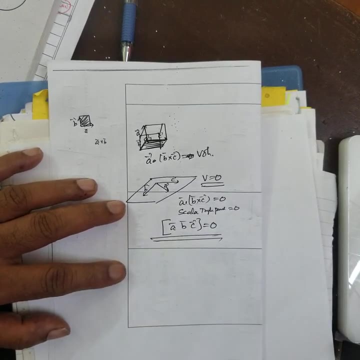 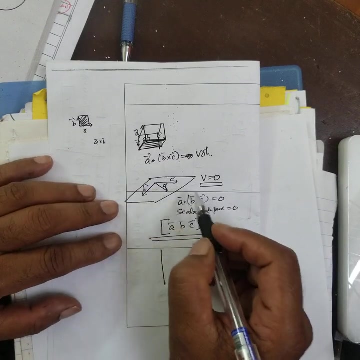 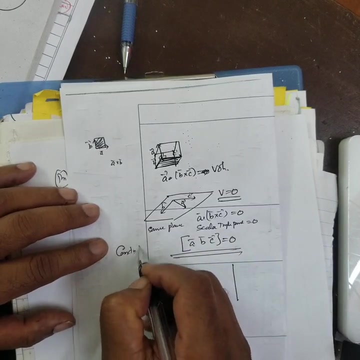 Triple product is equal to zero. This is called scalar triple product. Scalar triple product is known by A, B, C, equal to zero. Correct: Scalar triple product is zero. Now here: what is the condition for coplanarity? That means all three vectors are in the same plane. Same plane. What is condition for Condition for coplanarity? 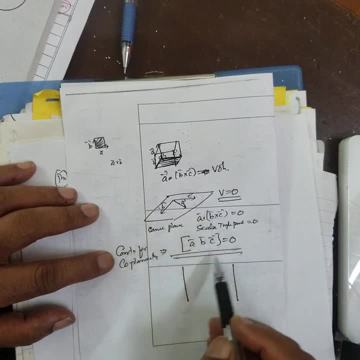 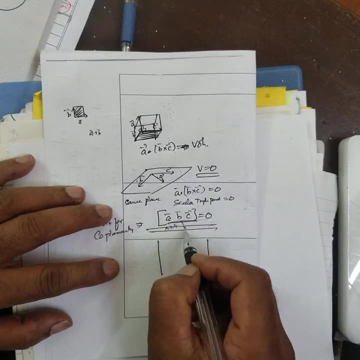 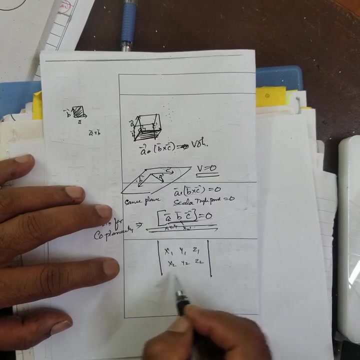 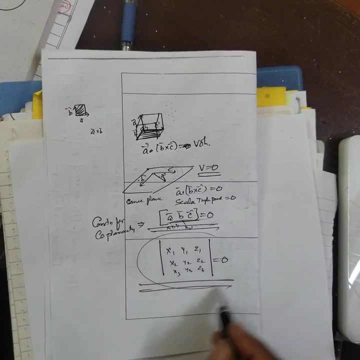 A, B, C are in the same plane, or volume is equal to zero, Or if A is equal to what, X1, Y1, Z1, X2, Y2, Z2.. We have started: X1, Y1, Z1, X2, Y2, Z2, X3, Y3, Z3 equal to zero. This is your circuit, right. That is condition for coplanarity. They are in the same plane, Same principle. I am going to apply it to the plane also. 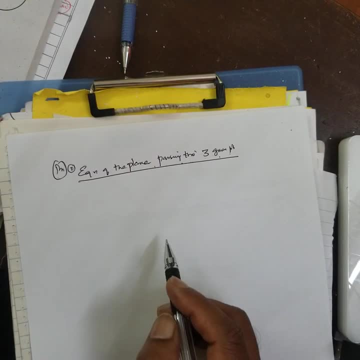 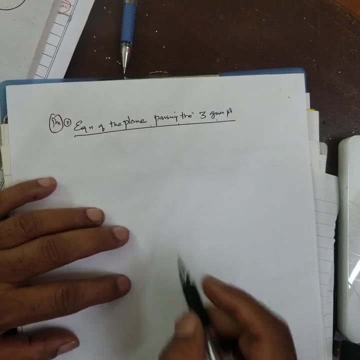 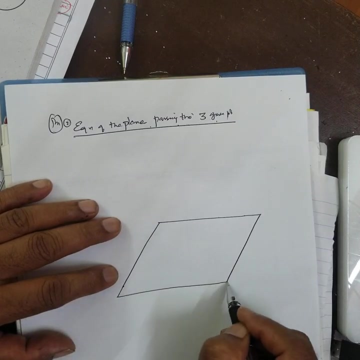 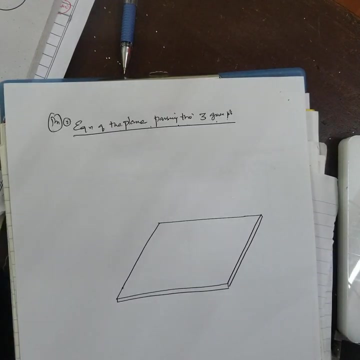 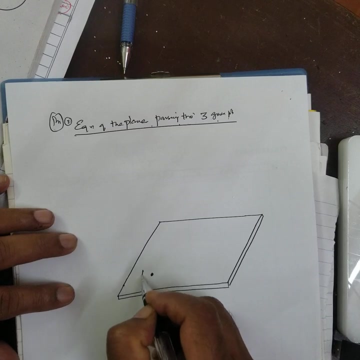 right now. consider a plane. consider a plane. here is a plane. here is a plane. in the examination you have to properly plan how to write the sentence right. consider as a plane now how i am going to start. let a, b and c. three points are the plane. that is what is a position vector? 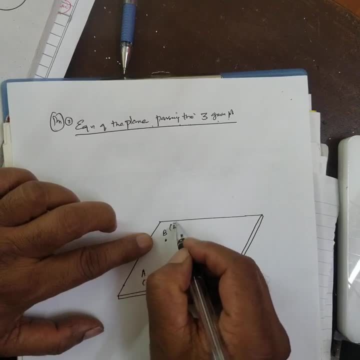 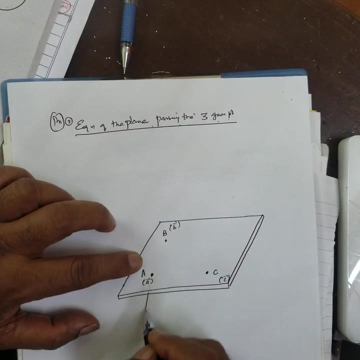 of a. is this position vector of b? is this position vector of c? is this that means here, here, here i'm joining right. this is a. this is b.